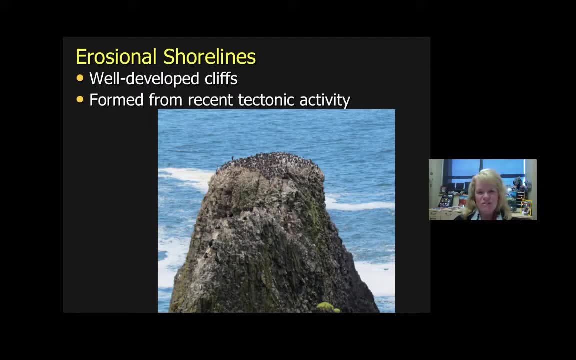 Greetings Earth scientists. We're going to learn about shorelines today, both erosional and depositional, and explain some of the features that you might see in the field as you travel. So if you're going to see an erosional coastline or 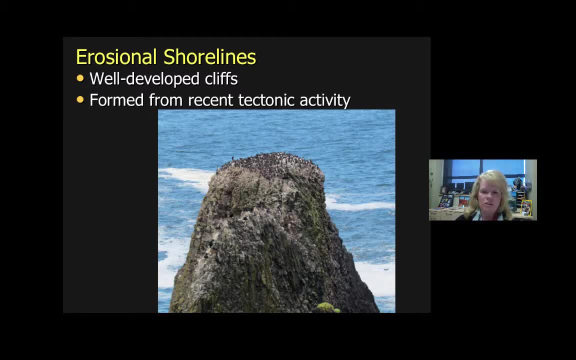 shoreline, you will see well-developed cliffs. I was on a sabbatical this summer and see all these birds right here. This is a big volcanic rock and they're using that as habitat because it's a volcanic sea sea stack where it's been eroded by. 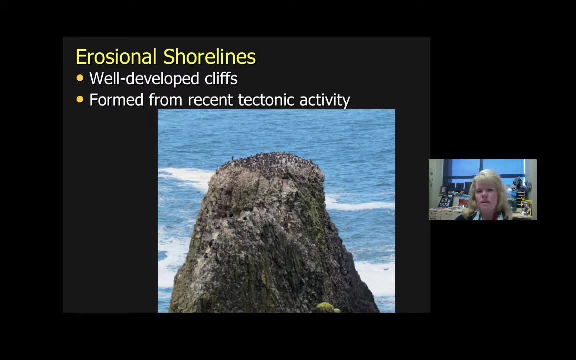 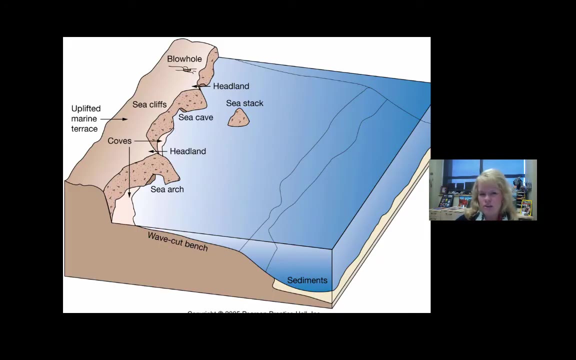 the water that you see behind it, which is the Pacific Ocean. So many of the erosional shoreline features you will actually see out in nature are pretty recently made rock. They're usually not very old rock. Some of the things you might see- A sea stack, just like you saw in the prior picture. You might see big 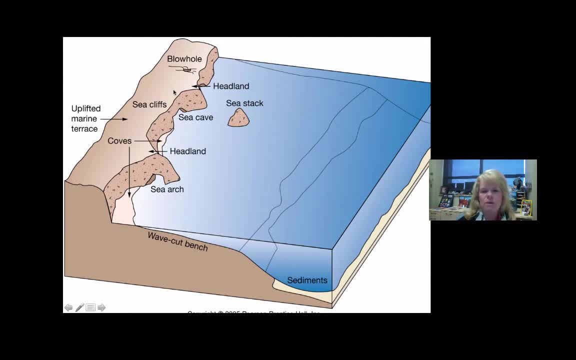 long, tall structures above an ocean area that would be called an uplifted marine terrace. Sometimes you'll see an area that's a cavernous opening in a rock where you'll get a blowhole. sea cliffs, sea caves, sea arches- All of these are features associated with. 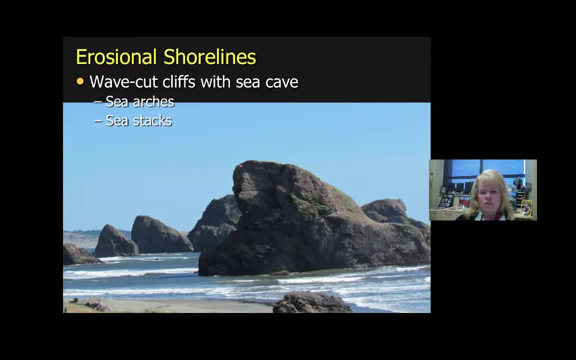 erosional coastlines. Here's a great look at what sea stacks looks like. There isn't even a sea arch in the background. It's kind of hard to see back here, but these are rocks that have been eroded by the pounding of water. 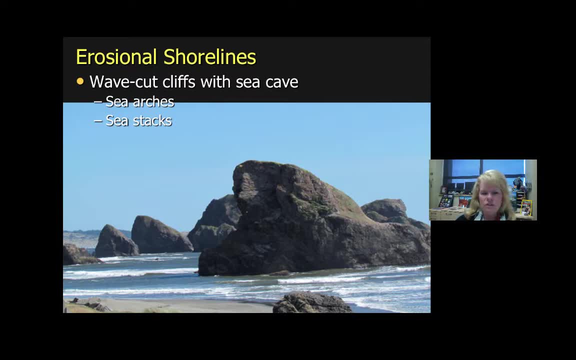 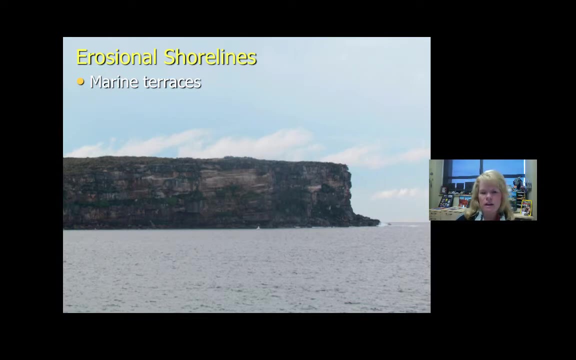 wave action 24-7. And so eventually sea arches will break into sea stacks, and so most some of these were combined as sea arches at one time. This is actually a marine terrace. that was I saw in Australia. This is in Sydney Bay. It's. 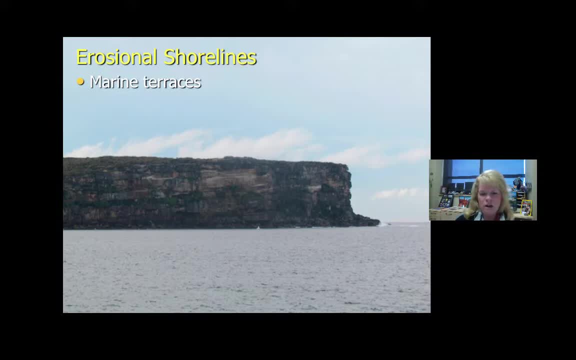 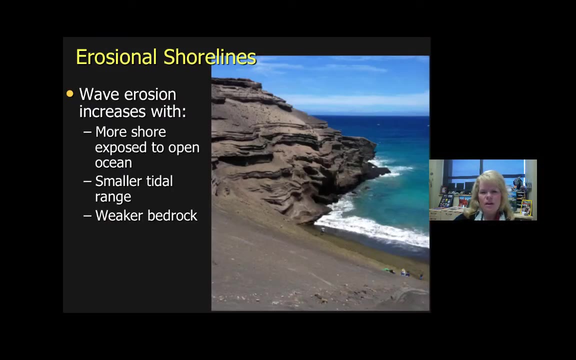 right where the Opera House is. I took a boat tour there and this is a big marine terrace and really quite interesting. the city of Sydney sits elevated up pretty high on a fairly large marine terrace that's made out of sandstone. Sometimes a wave erosion will happen at different rates for different types of rock. That's. 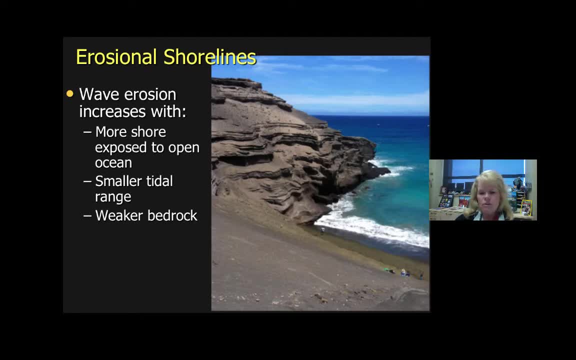 called differential weathering. This is actually one of the most beautiful beaches I've ever been to. It's called the Green Beach and Green Sand Beach. that is at South Point on the Big Island of Hawaii And it is very remote to get to. The green actually comes from peridot, which is olivine, the mineral 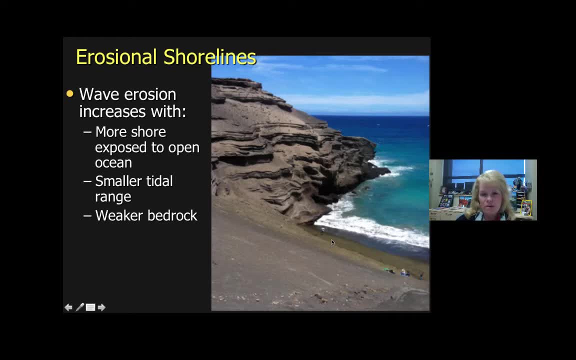 olivine, which has to deal with the mafic rock. If you remember about learning in rock cycle, about igneous rocks and the dark rocks that we have that are called mafic, that's an example there. So this is a small embayment area. It's cut. 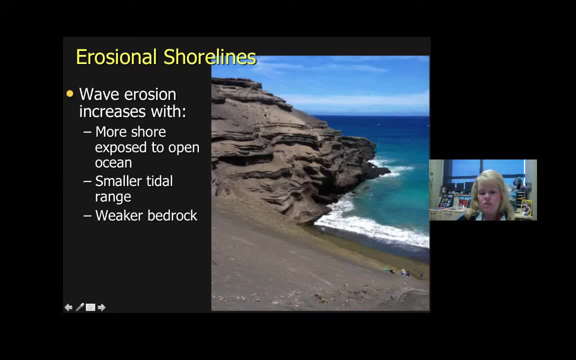 out one section pretty well, but these have not. these layerings of lavas and ashes have not weathered as quickly. The more open the area is, the more likely it is to impact wave action, the more likely it'll erode faster. So there's. 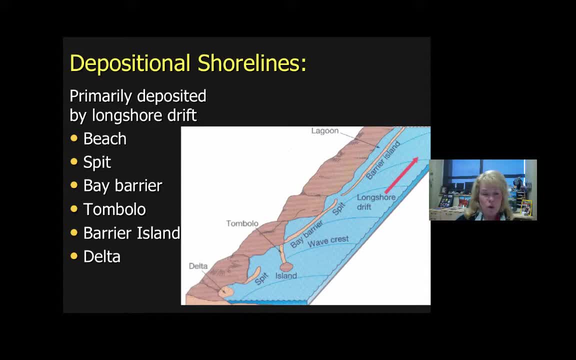 some depositional shoreline features as well. Let's take a look at some of them. Of course there's beaches. You might go what's a spit You're fixing to learn out. learn what that is: A bay barrier, a tombolo- which is one of my favorites- a 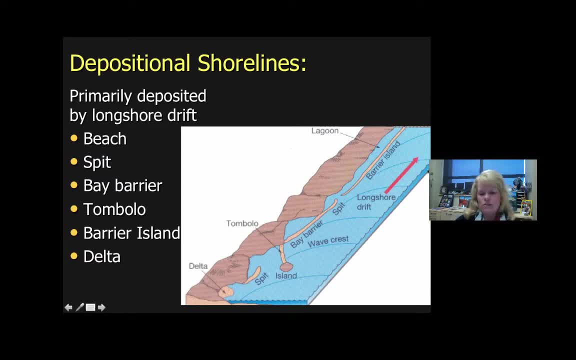 barrier island and deltas. So we're going to take a look at each of these features. You can just see this is a spit right here. This is where you get the beginnings of a barrier island. A barrier island is, or a bay barrier is, one that grows across the entire bay. 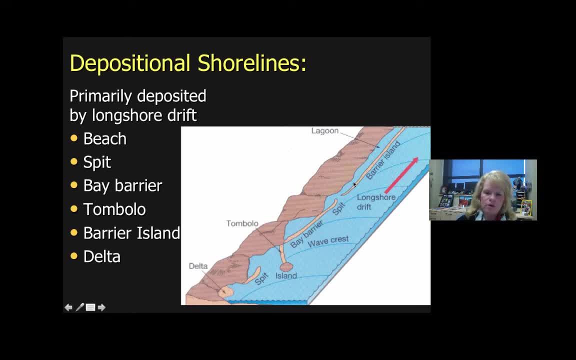 region. A true barrier island is going to sit further out and have a lagoon behind it. This is a little bitty spit right here, but when you get a spit that grows out and has some kind of rock that waves have wrapped around and deposited, 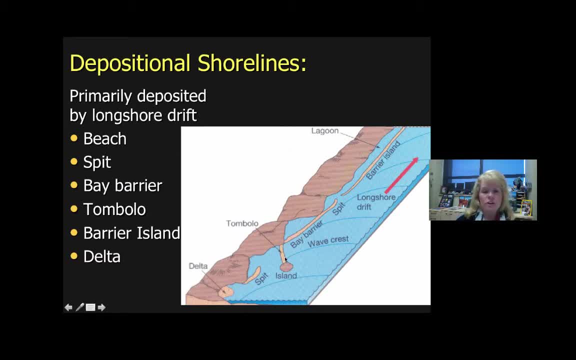 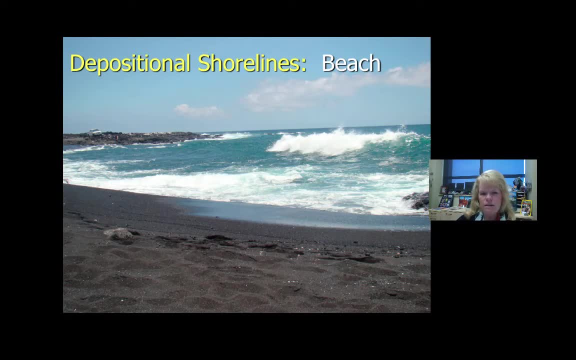 sediment behind it. that's called a tombolo. So let's look at some of these features and show them to you. This is a black sand beach in Hawaii. as I was walking back from the green sand beach, This was what I walked on, And 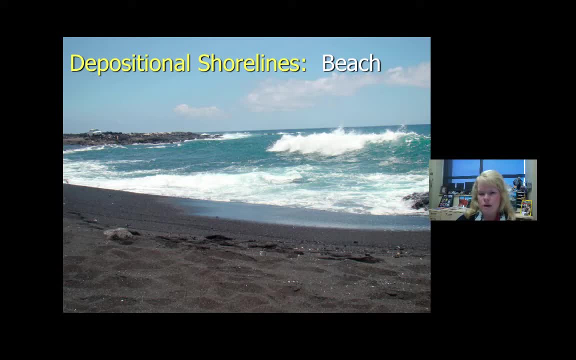 beaches are not made by accident. They're made from whatever bedrock hits is being hammered by the shoreline. This is almost exclusively black and green sand, with just a little bit of carbonate, fossil material or rubbage from living material that's recently died. 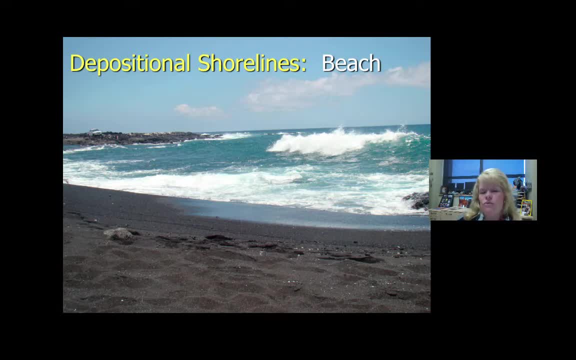 I know that because the instructor I took a course, several courses from that- does work in Hawaii beach sediment studies of Hawaii And I actually looked at the percentage of black sand, green peridot, olivine white, which is the carbonate material to 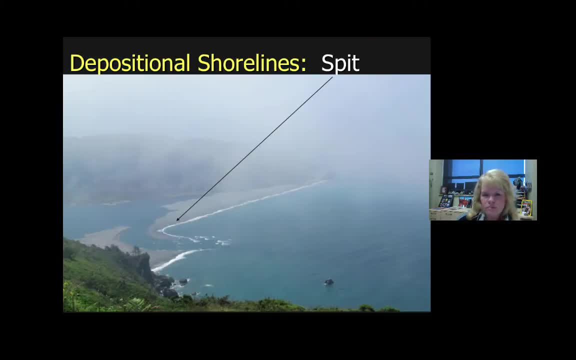 determine the ages of the beach. This is a spit. I saw this in my travels this summer as I was traveling from the Redwood National Forest up into Oregon. It was a really foggy morning, but if you look you can see where deposition has. 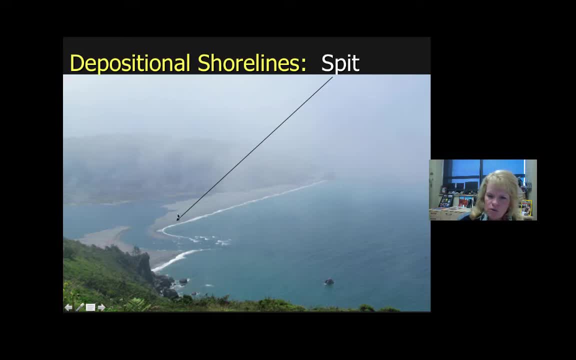 occurred from long shore currents right here And we've almost got a full barrier- bay barrier- situation, but it hasn't grown all the way across. Until it grows completely all the way across do you have a bay barrier. But this is a classic spit, This is a 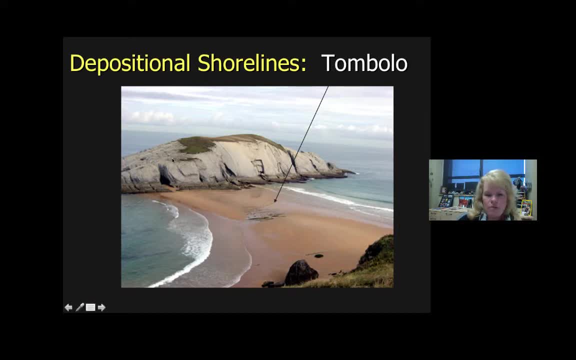 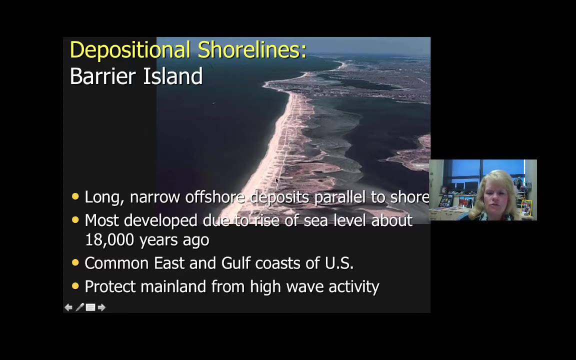 classic tombolo. So you have, this rock acted as a barrier, and so the currents are going to hit this, wrap around the rock and then deposit sediment behind it. A barrier island is where you get a formation of a long stretch of spit. 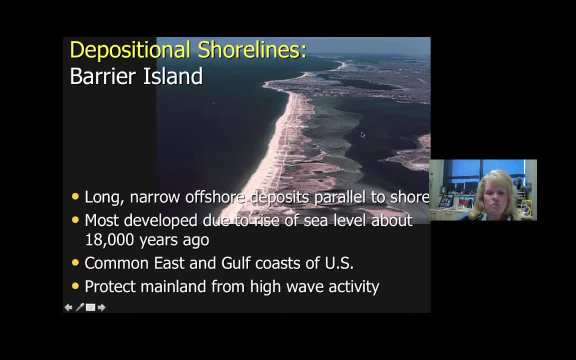 material that actually hooks together and makes a lagoon behind it. Most of barrier islands around the world are fairly young in geologic age and most of them formed at the conclusion of the last ice age. Very common that we have them on the East Coast and in the Gulf of Mexico, One you might be most. 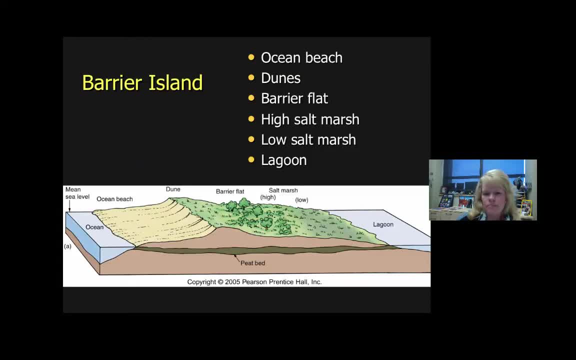 familiar with is Padre Island. Barrier islands can produce interesting situations where on one side you have a beach and the other side you actually have marshland material And that has to do with the side that's getting the ocean, derived currents and then the side. 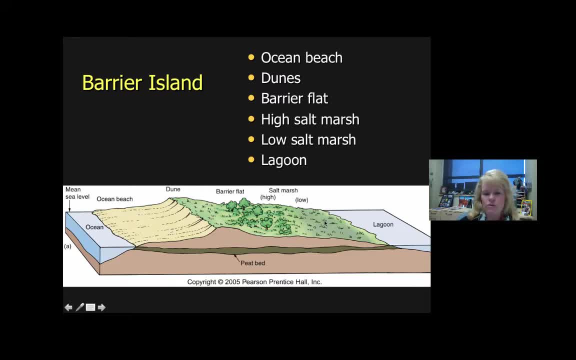 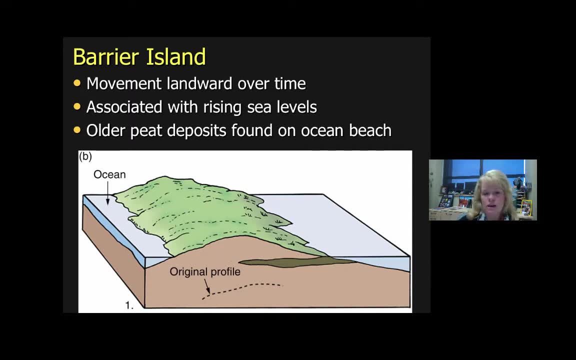 that faces the lagoon, which is going to usually have more moisture. A barrier island can move landward over time and eventually join with the land. They can be associated with rising sea levels, and the oldest deposits on the ocean beach will tell you the age of the island, and that'll be. 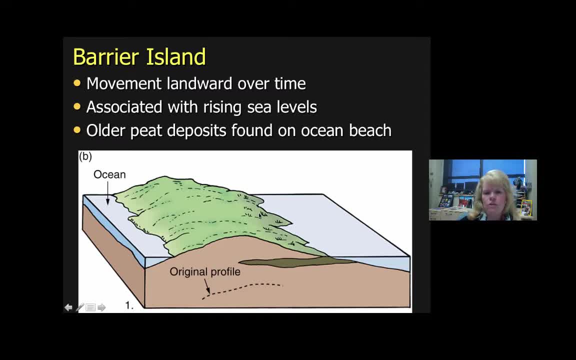 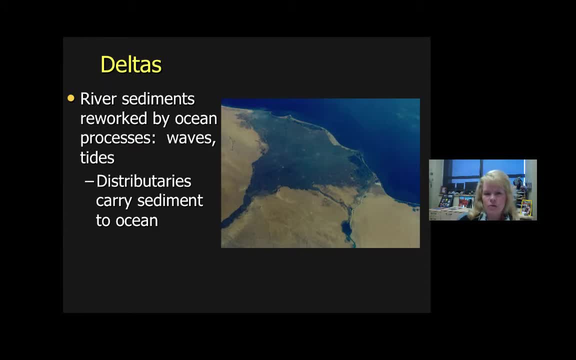 the dead marsh material that turns into peat, which is the beginnings of coal formation. Deltas are river sediments that get reworked by waves as a river enters in a water body like an ocean, and it carries sediment into the ocean in the form of teriginous material. This is a delta I saw in Olympic National Park. 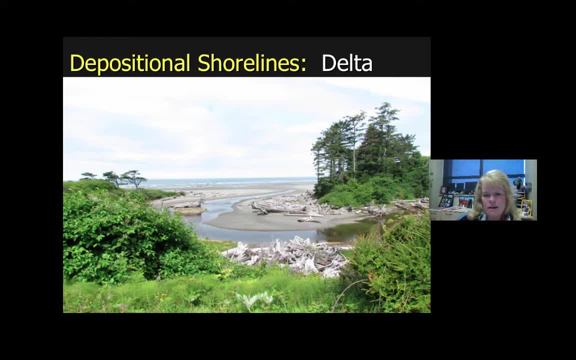 For those of you who are fans of Twilight, I showed this same picture to you a little earlier in one of our lectures, and this is actually where water is feeding into an ocean and making deltaic deposits here. This is in the same area where Forks is located. if 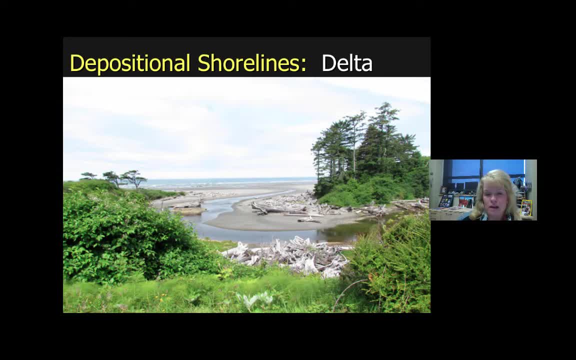 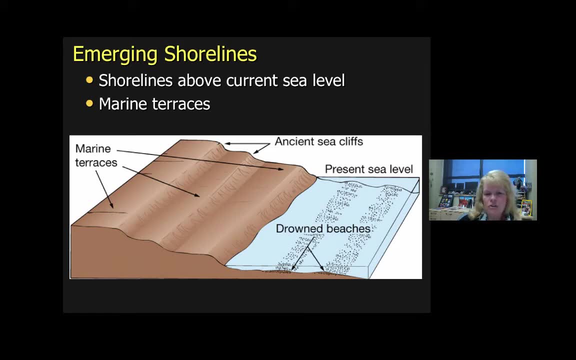 you guys are familiar with the city of Forks from the Twilight movies. Emerging shorelines are those that represent terraces that are now above sea level that used to be a shoreline. There could be several reasons this would happen. One is sea level has dropped, obviously. Another is 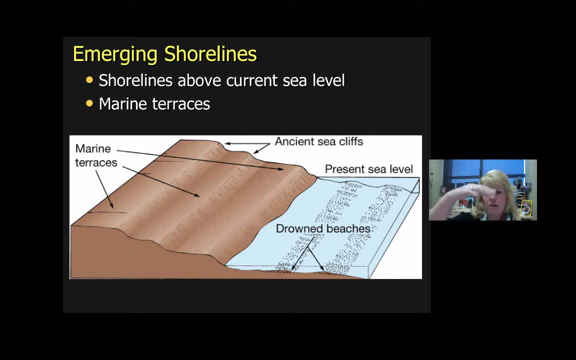 isostatic rebound where the ground has popped back into place. I can still think of a third reason. There's a couple of places like this in Alaska where in an earthquake that happened in 1964, a bunch of land got shoved upwards, and when it 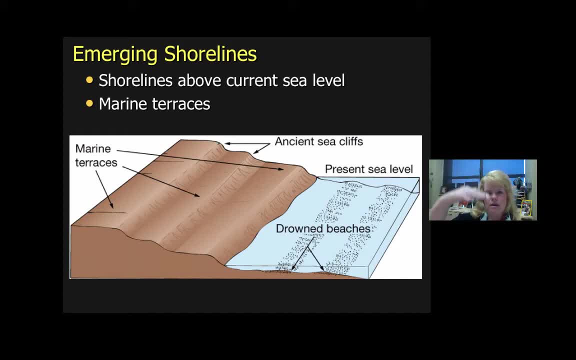 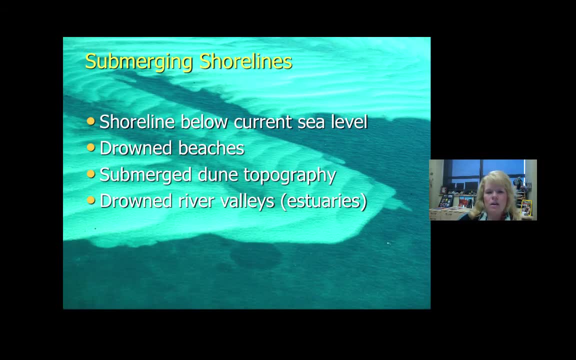 did. the beach line deposits were moved up about 30 feet and the new shore line is making a deposition of a beach in its current location. So submerging shorelines tell us that these are shorelines that are currently below sea level. that used to be the shoreline. Essentially, they are. 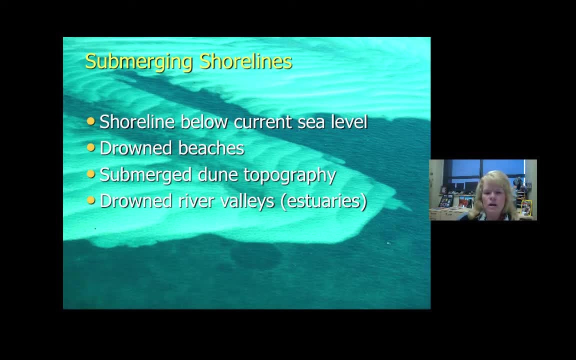 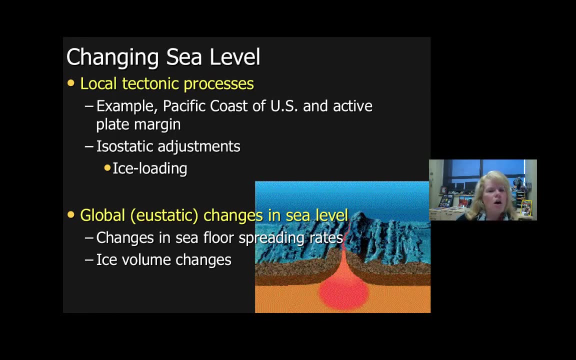 drowned beaches that are now covered by water and they make dune-like topography, like you see here in the Bahamas. What can cause these sea level changes that can create submerged or exposed elevation, sea level or sea marine terraces. It can be local tectonic processes, like I. 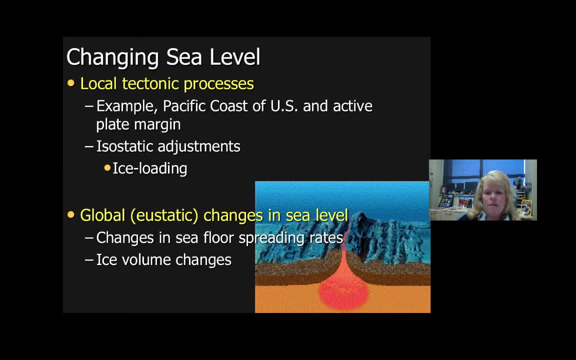 mentioned with the Alaska earthquakes, isostatic rebound from where mountains have eroded down and the ground pops back into place. The same would be true with glaciers. We can also have a worldwide eustatic sea level change. Maybe that's from active mid-oceanic ridge activity, like you see right here. 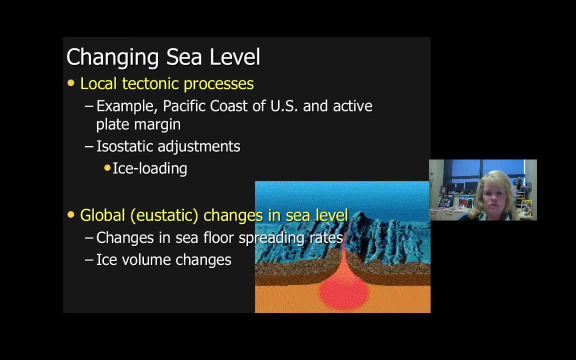 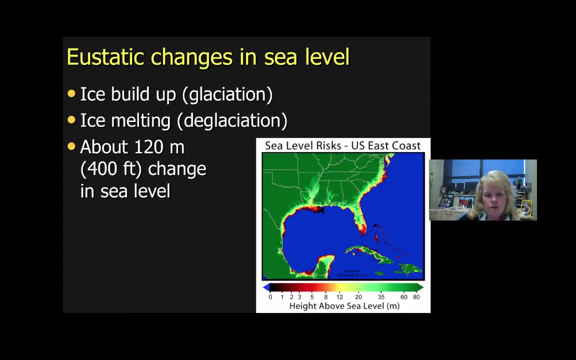 or even glaciation changes at the North or South Pole. Eustatic sea level changes really are very closely associated with climate change. When we're looking at ice buildup, we're talking about glaciation in the form of massive continental ice packs and sea ice In the last ice age sea level. 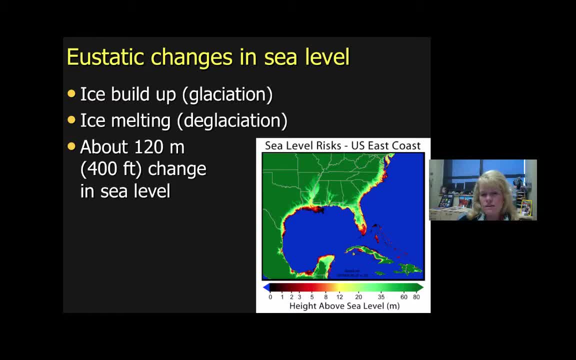 dropped between 300 and 400 feet. 300 to 400 feet, that's incredible. So as the ice packs begin to melt, sea level will gradually rise. That's very significant because these areas in here are highly populated regions where people live, so there has to be a place to put those people after. 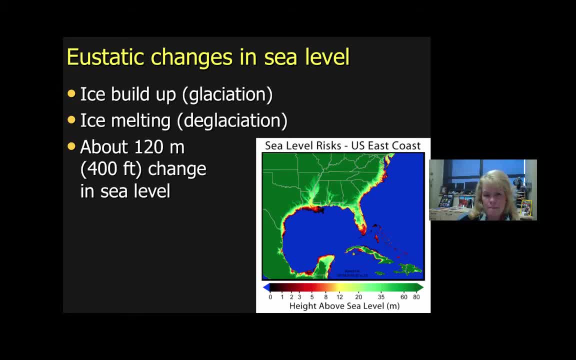 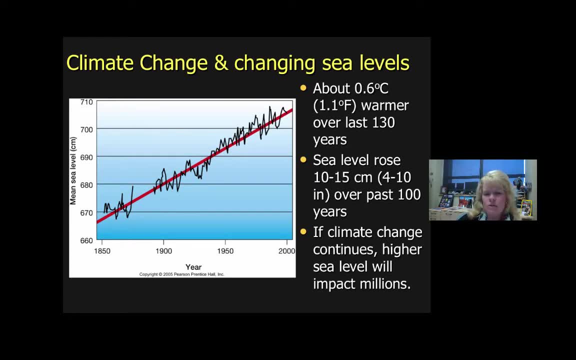 sea level rises over a period of time. Climate change and changing sea levels are a pretty hot topic. We've literally over the last 130 years have risen a little over 60%. Sea levels have been growing. We think sea levels are a. 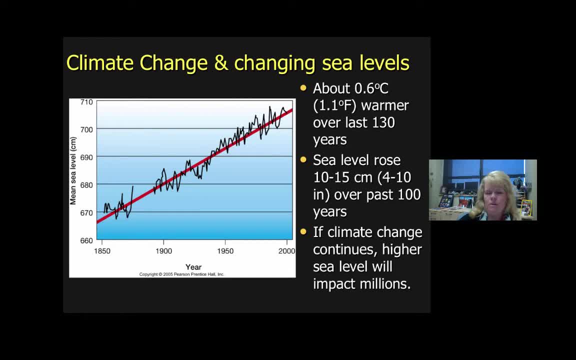 a degree Fahrenheit. We'll be talking more about climate change in our last lecture. That's a scary thing, because if sea level continues to rise by 10 to 15 centimeters- that's like a foot over the past hundred years- that's going to begin to flood people's homes out, So we will expect millions of 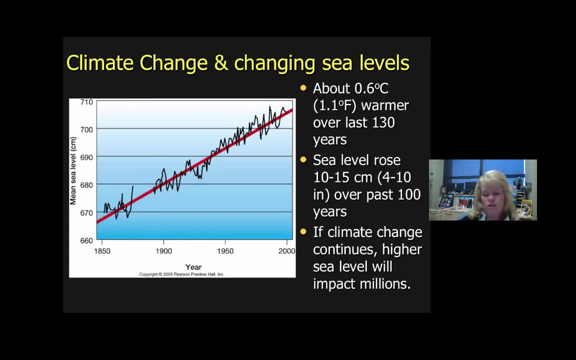 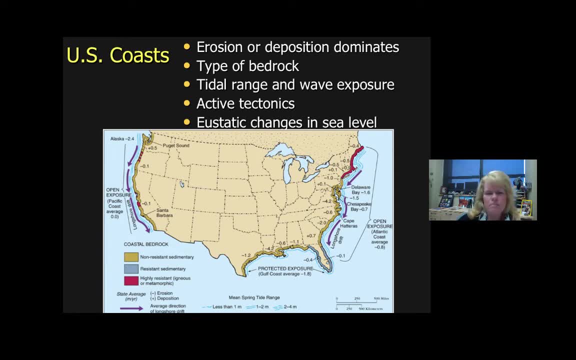 people to be impacted by that long-term trend. Our US coast have two different types of personalities. It's going to be based on the types of currents that come in, specifically the bedrock that's being impacted by the wave action and the amount of tidal range that's in. 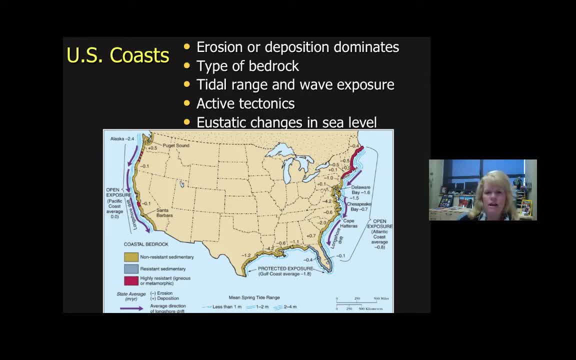 that area? Also, is it a passive or is it a active continental shelf? So let's take a look and see what those areas are. On our US coast we have some interesting situations where we have bedrock that's different throughout the United States. A lot of that's. 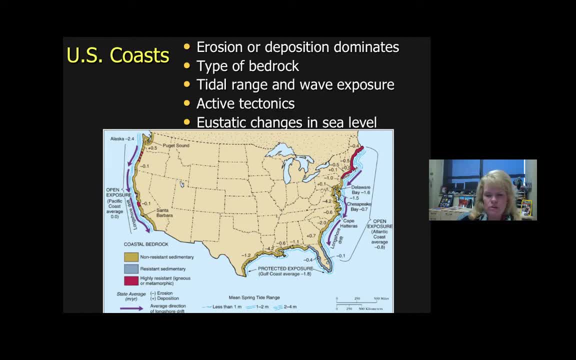 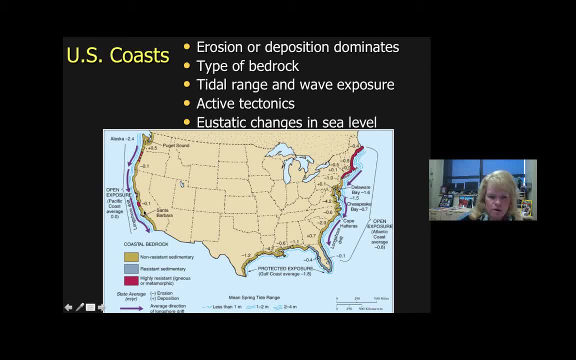 the Gulf Coast and most, but not all, of the West Coast, you'll see that it's nonresistant sedimentary rock That's going to break down pretty easily. You get a couple of patches of red here, a couple of red patches here and a significantly patch right here. that's going. 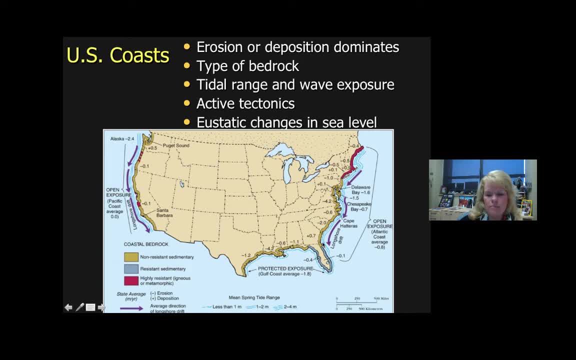 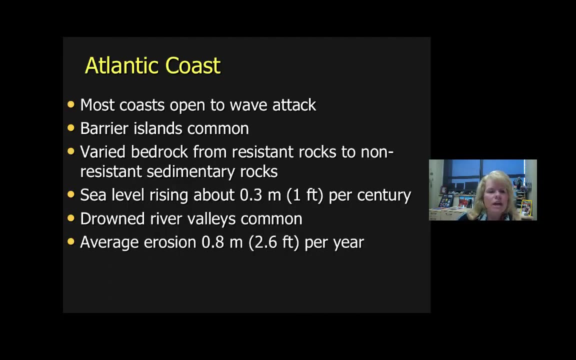 to be highly resistant: igneous or metamorphic rock. Down in this blue section, right here, you have pretty sturdy hard sedimentary rock, usually in the form of dolomite or some kind of hard sedimentary rock that doesn't weather very fast. So let's take a look at the Atlantic coast- Most of the coasts. 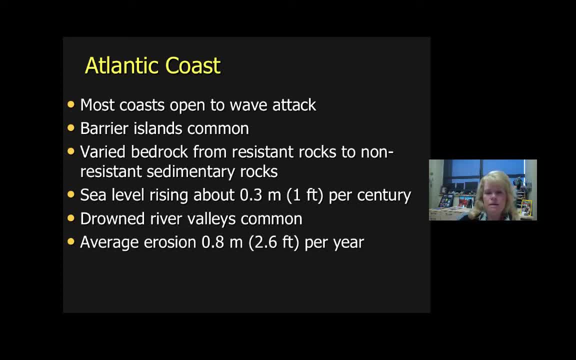 are just ready to be bombarded by wave action, and that's why we have a number of barrier islands common. The bedrock is completely variable, from softer rocks to not so soft rocks, and literally we've seen that sea level rise by a foot in the Gulf of Mexico in the past century. So we definitely have 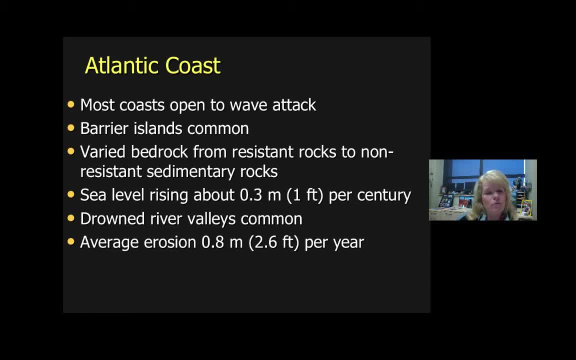 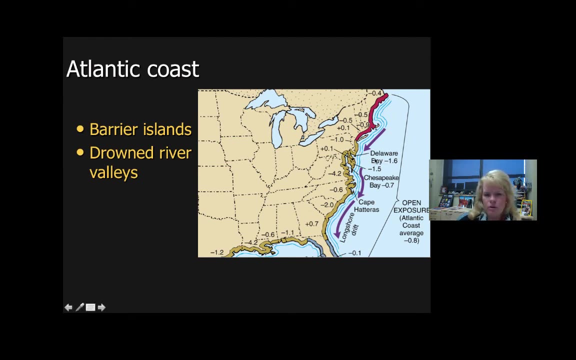 drowned river valleys that were present in those areas from the last ice age, and the average rate of erosion of these rocks is literally 2.6 feet per year a bedrock. So along the Atlantic coast, you would expect to see barrier islands around the Atlantic coast. So along the Atlantic coast, you would expect to see 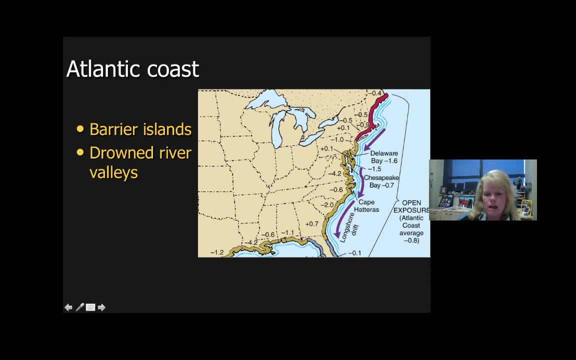 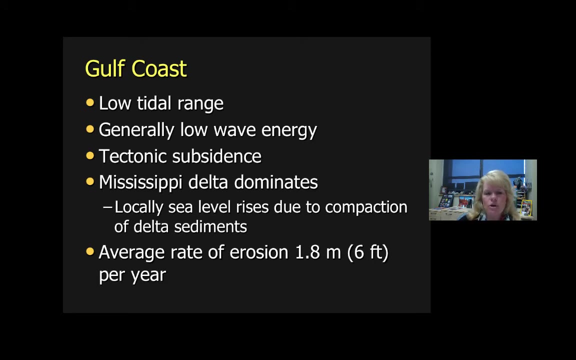 here and in this section and drowned river valleys, The not so soft rock which would be the blue areas around Florida and up here in the New England states, you would expect to see different types of situations occurring. The Gulf Coast has a low tidal range, has low wave energy, which is one of the reasons you 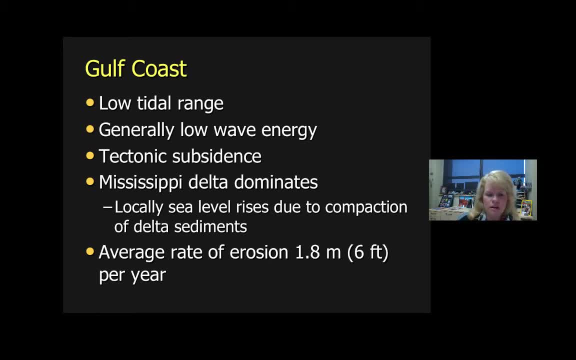 don't see too many beaches of significant nature. We actually have subsidence happening in the area, so sea levels actually dropping. if you have an area that's compacting a whole bunch of sediments from deltaic deposit, it may actually show that the sea level is rising a bit- The average. 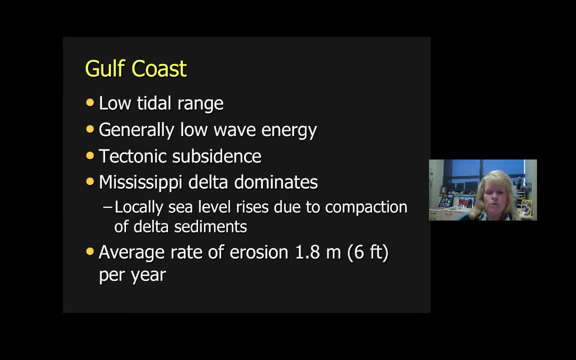 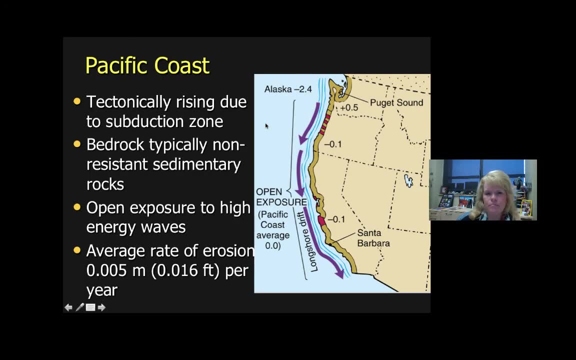 rate of erosion in the Gulf Coast is six feet per year. So that would be this region, and here it's losing mass instead of gaining. The Pacific Coast is extremely active shelf. right here you have a subduction zone and this section is the Pacific Coast. 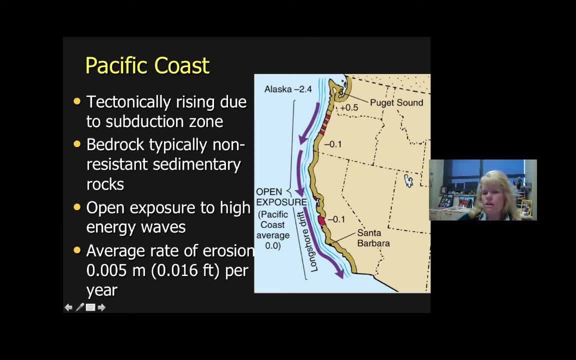 You have the San Andreas Fault. The bedrock is typically not sedimentary. that are very resistant to erosion and if you have sedimentary they are non resistant so they tend to erode pretty quickly. You'll have a lot of beaches along that area If 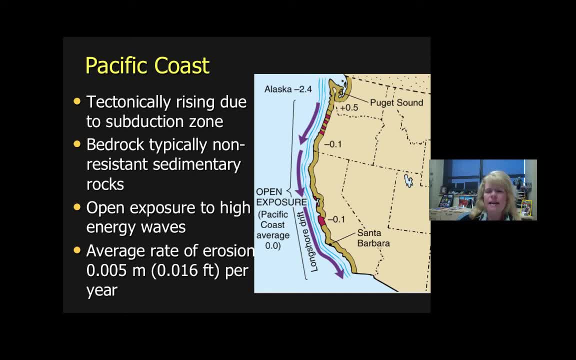 they're not that way. they may actually be igneous, and then you could actually have a lava where it would break down and make interesting features like sea stacks, sea caves, especially from this area and right in this section, right here. The average rate of erosion here is 0.016. 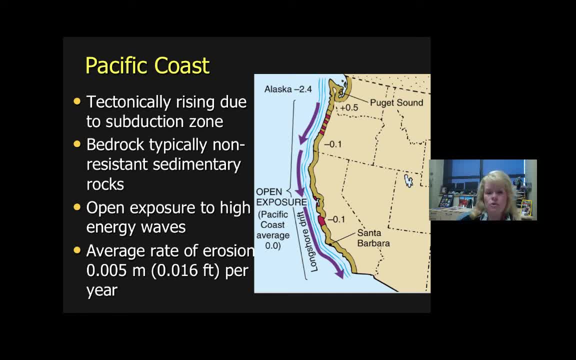 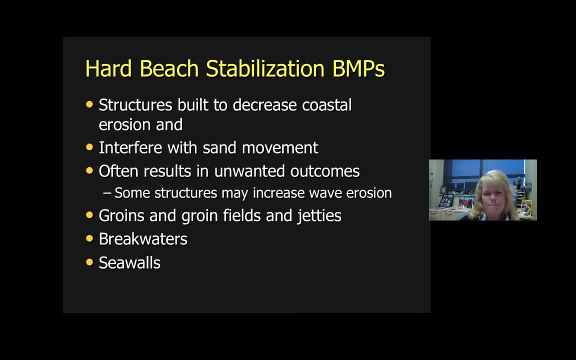 feet per year, indicating the rocks are more durable. There are beach stabilization BMPs As a test question. what does BMP stand for? Best Management Practice? These are structures that are built to decrease coastal erosion and help with the interference of sand movement. They often result. 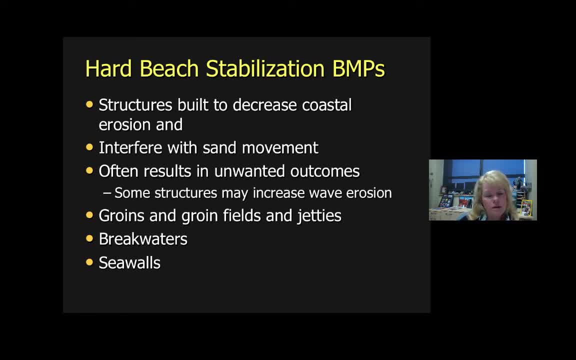 in unwanted outcomes. Unfortunately, we can't stop Mother Nature from doing her thing, So there's a couple of them that we're going to learn about. They're grow-ins and grow-in fields and then jetties, And these are all best management practices you might see in a coastal area. 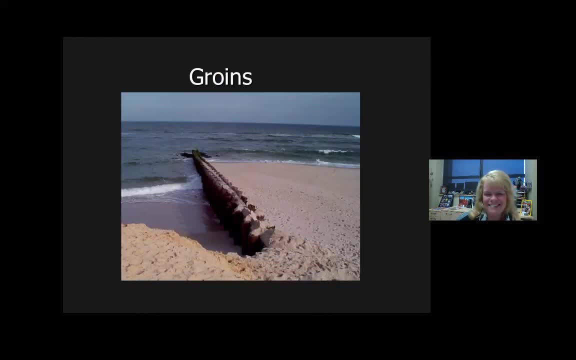 breakwaters and seawalls. So let's take a peek. This is what a grow-in is. You might have called this a jetty in your past, but grow-ins are singular features and there may be a number of them in a row along a beach line. 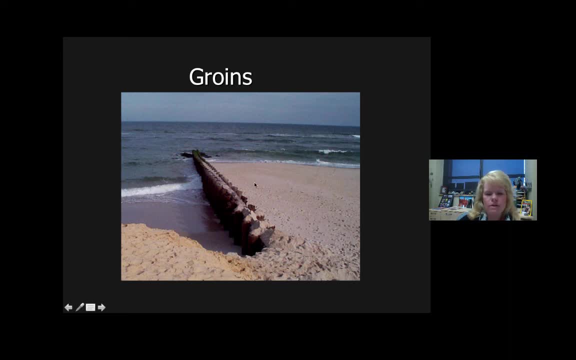 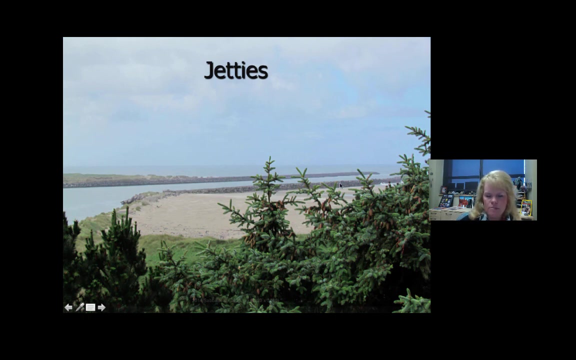 The idea is to stop beach drift from longshore currents, but you can see they need to come in and pull out some of the sand and move it back so this thing doesn't get destroyed. A jetty has two of these structures like this one in Oregon. I was in Newport, Oregon, this summer and I saw this shot. 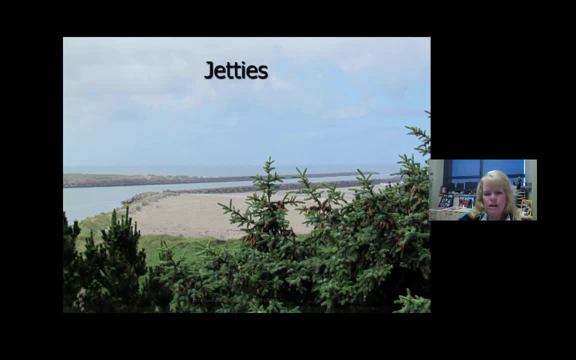 and I was like, wow, look, there's a great jetty And this is a jetty has. it's almost like a street that you've built with a. they're light grow-ins, but they're two of them And this is a jetty that.